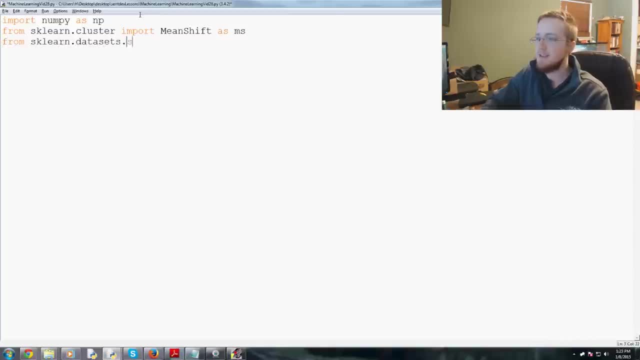 Then we're going to go ahead and import numpy as ms. So what we're going to go ahead and do is: from sklearndatasetssamples underscore generator import, make underscore blobs. So what we're going to have to do here is we're not going to be able to be using the same dataset that we've used up to this point for a sample. 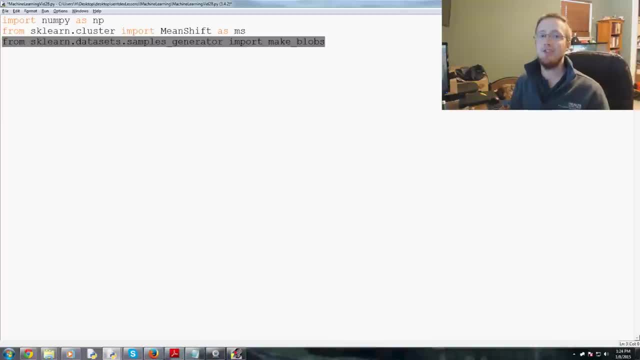 Because it only has six data points, And six data points is too few data points to use with mean shift. It's really too few to use anywhere, But it's It just worked for us up until this point, But it's not possible to do it with mean shift. 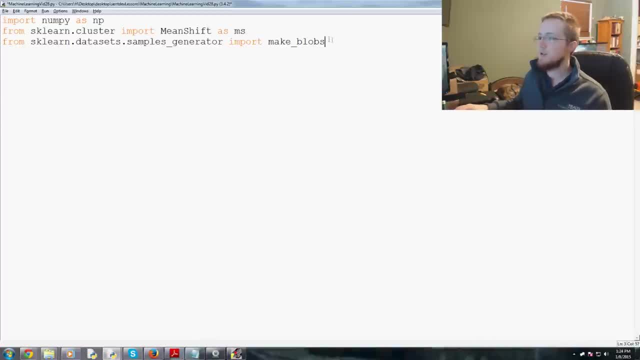 So, anyways, we're going to make our own sample, And what this is going to do is it's going to Exactly what it sounds like. It's going to make blobs of data based on standard deviation, a little bit of randomness. It's going to make blobs of data around a point that you specify. 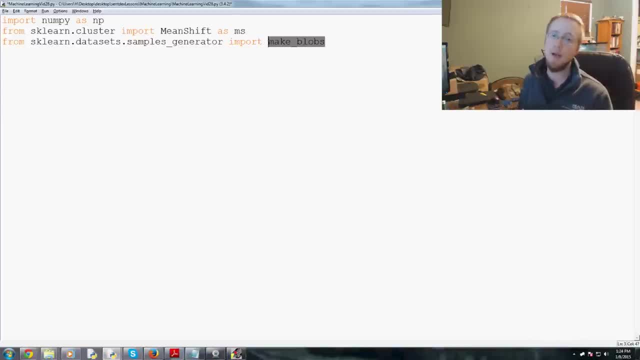 And you'll say how many data points you want around that point, And then also you can specify the standard deviation. So that's what we're going to use that for. And then, finally, We're going to import mapplotlibpyplot as plt so that we can actually visualize our data. 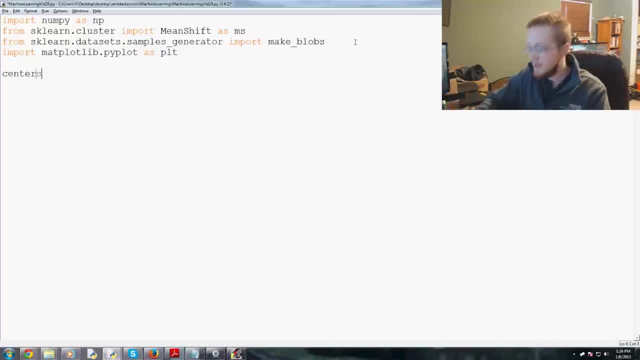 So now we're going to go ahead and say the following: We're going to specify a centers variable And it's going to be a list of lists. Now, for now, we'll just have two data points. to start with, We'll use a 1 and a 1.. 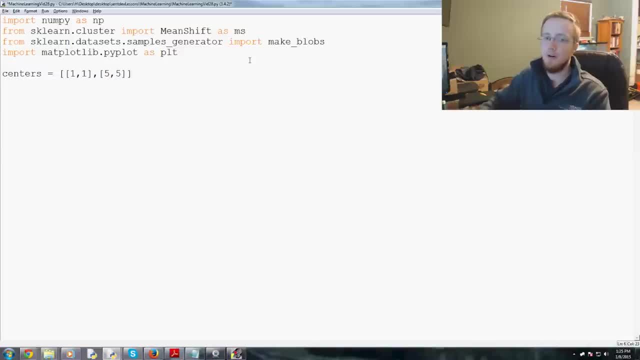 And we'll use a 5 and a 5.. So those are our center points. Now we're going to specify x and a lowercase y, And if you happen to see any other tutorials on this topic, you may see people do x underscore here. 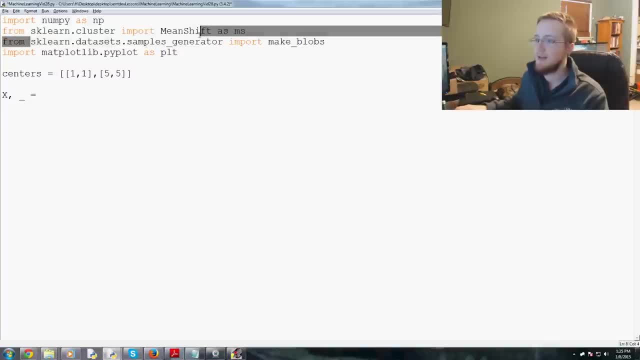 And the reason why they're doing that is this from sklearn dataset sample generator. What it's going to do for you is actually two things: It generates sample data, but not just any sample data. It's specific to machine learning And it's generalized data for either unsupervised or supervised machine learning. 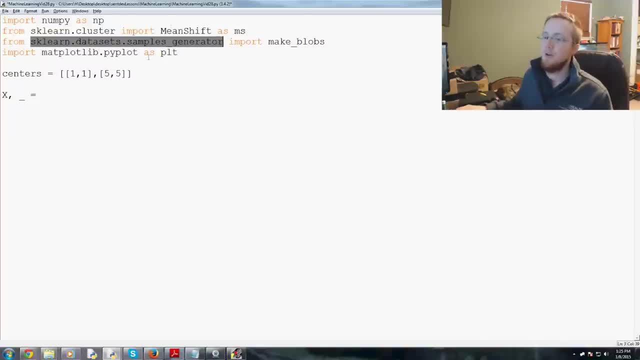 So what it's going to do is: it's going to come. It's going to come with labels. So whenever you see this underscore like this when we're unpacking variables, it means pay no attention. It's useless in this example. basically. 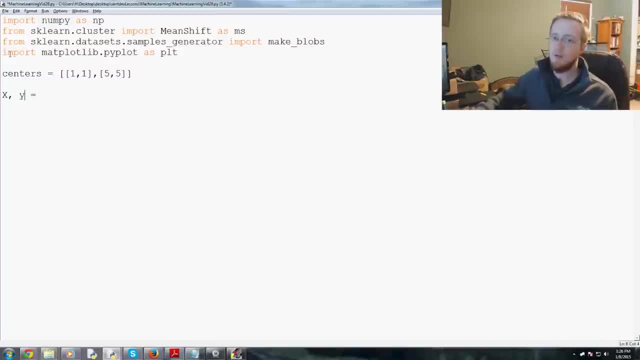 I'm going to call it y because that's what it is And that's how it relates to the other videos in the past. But just understand that the reason why people might underscore it is to kind of underscore the importance of understanding that normally you do not have labeled data. 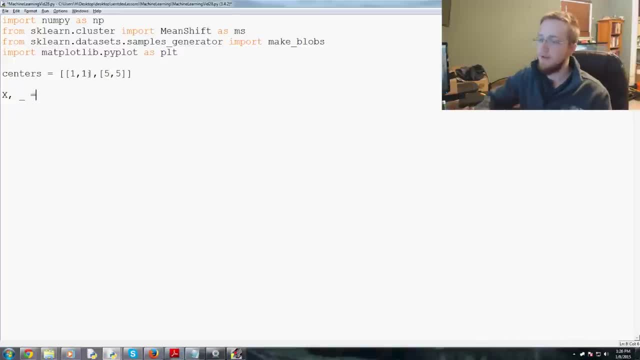 So I don't know, Maybe I'll just leave it there. actually I don't know, It doesn't matter, Just understand what that purpose is. So anyways, make blobs. I love that joke. Underscore, Oh man. 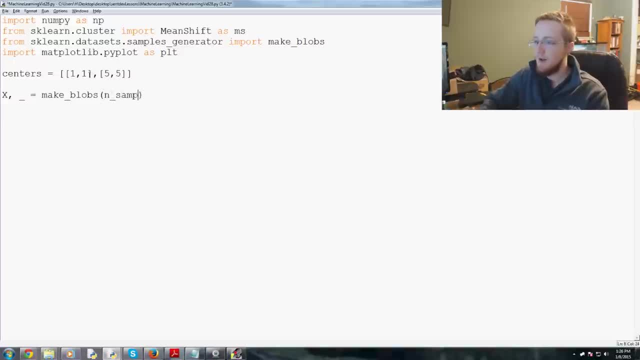 So funny. And to make blobs. you're going to say how many blobs you want, So n underscore samples. This will be how many blobs do we want to create? Let's make 100.. Just for the record, mean shift is thought to be accurate up to 10,000 samples. 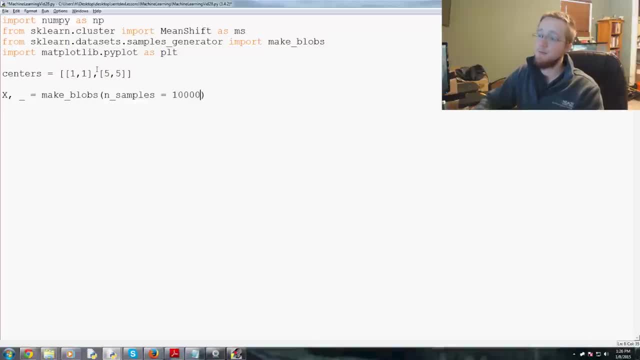 More than that, you're in trouble. So if you have data that's bigger than 10,000. 10,000 samples- you're going to need some way to simplify that down. You can actually use machine learning for that specifically, even unsupervised machine learning. 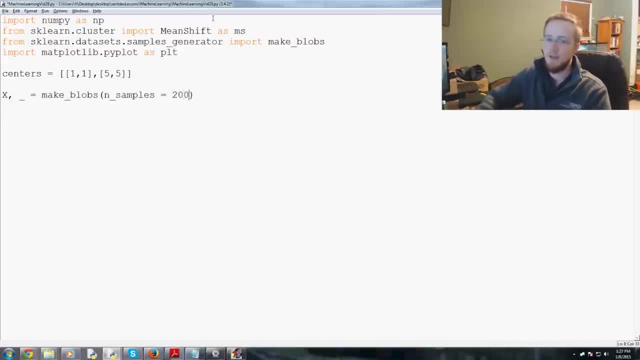 but maybe more on that later. For now, our number of samples, we're going to say, is 200. Then centers is going to equal well centers, And then finally, cluster underscore standard deviation is going to be 1, for now. 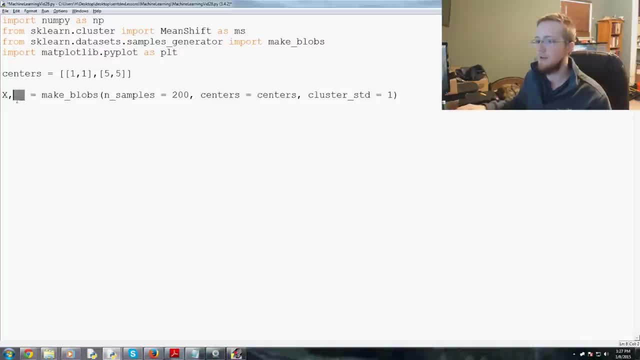 So this is our function: we're unpacking to a variable that doesn't matter and, of course, x, which is our data set. Now what we can do is we can do a pltscatter and we can scatter using that fancy code that we learned. 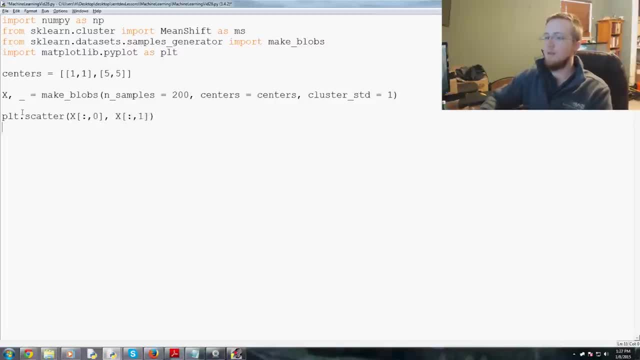 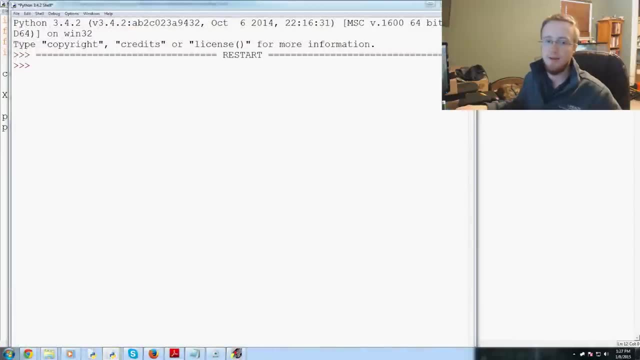 So capital X, colon, comma 1.. And then finally run a pltshow on the data Whoops, And we will save and run that, And here we have our lovely. This is the data set that you know with your eyeballs. you can say: 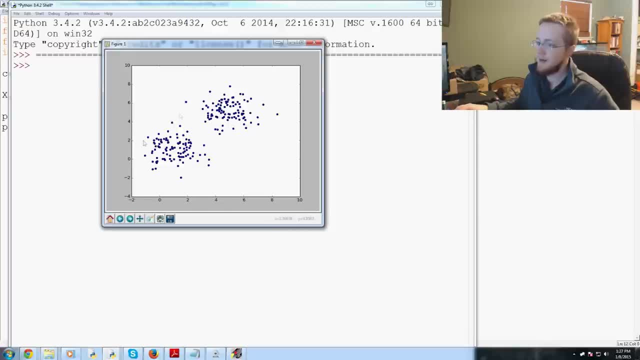 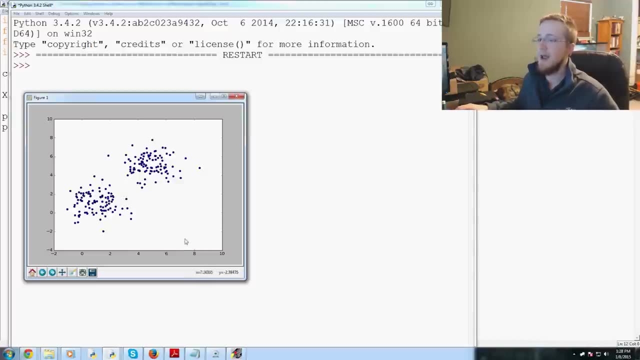 okay, this is a cluster here and this is a cluster here. Now we want the computer to make that choice and we're hoping that it really does indeed say: this is a cluster and this is a cluster. and it doesn't say: well, here's a cluster here and here's another cluster. 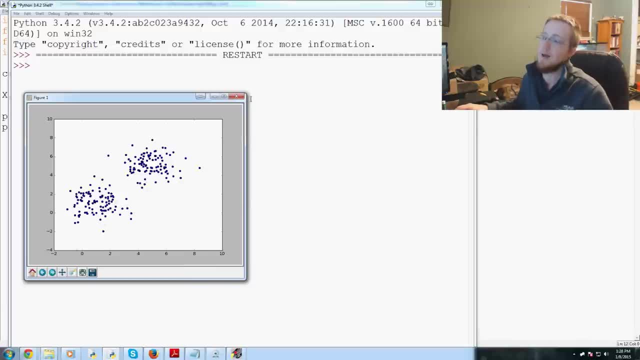 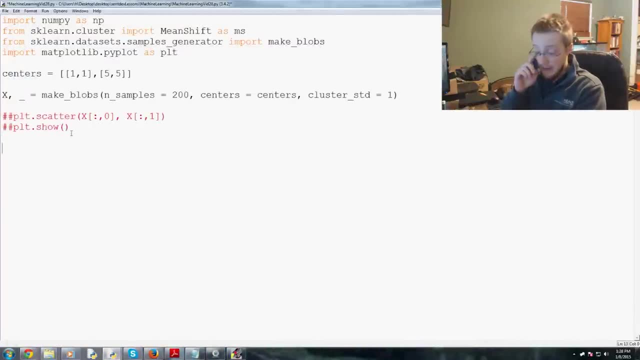 and another cluster. and then here's another cluster. We don't want that. We're hoping it doesn't do that. So anyway, closing out of this, I'm going to comment this out. We don't need this anymore, but if you want to look at it, that's totally fine. 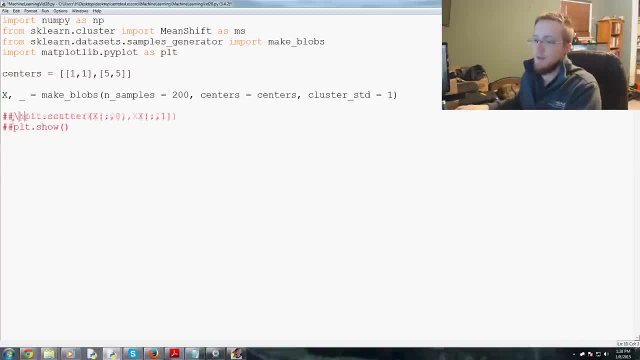 Now, And in fact maybe I'll leave it up for the first time running, because it'll be a scatterplot of the same data, non-colored because we're going to end up coloring it Now. we're going to reference ms for mean shift. 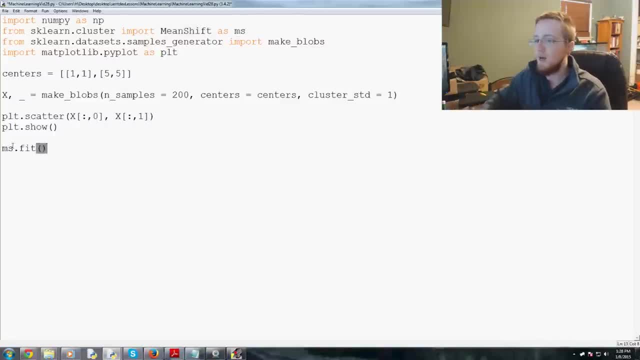 So now we're going to say msfit and we're going to fit a capital X there. Now what we're going to say is the labels equals, mslabels underscore. Now, please don't confuse these labels. These are the actual labels that were used in the generation of the data set. 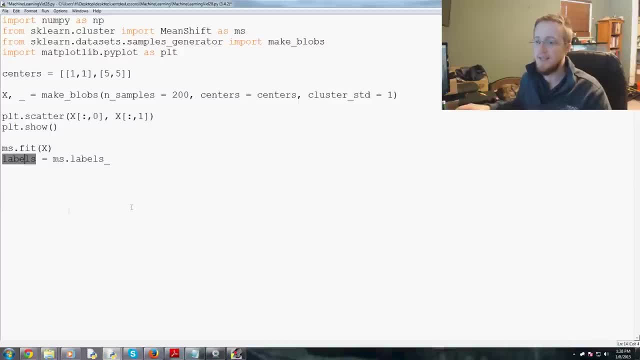 These labels are the labels that the machine has assigned to the data. So later on, of course, you could compare these labels to these labels, But I will just say that that might be useless as far as generating any sort of performance because, for example, if we put these two centers close enough, 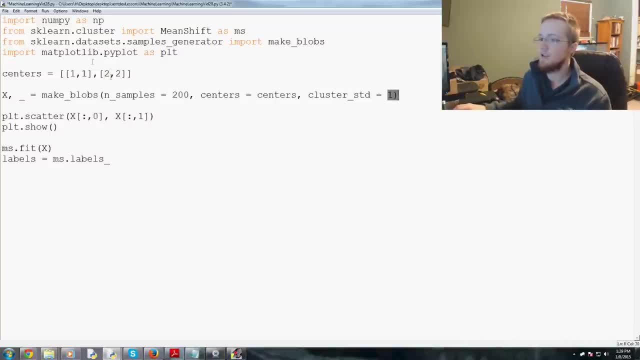 like, say, we generate with a 2 and a 2, standard deviation is 1.. Therefore, we're going to have some cross-references, We're going to have a crossover that could be justifiably so, more related to this than this. 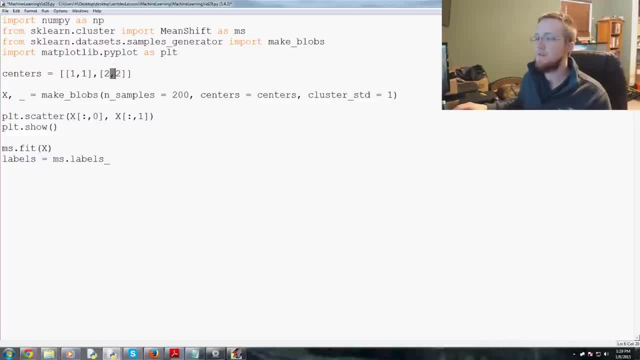 That's just the case. So just keep that in mind that if you've got enough standard deviation in your samples- even if they come pre-labeled- and then you're using that to test your unsupervised clustering algorithm, just understand that it's going to do what it thinks is best. 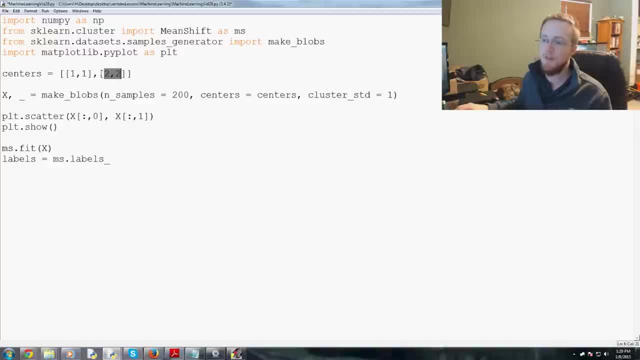 And if the data, even though it was generated with an initial 2,, 2,, if the variance is enough, it makes more sense to be clustered with the 1, 1.. So keep that in mind Moving along. those are labels. 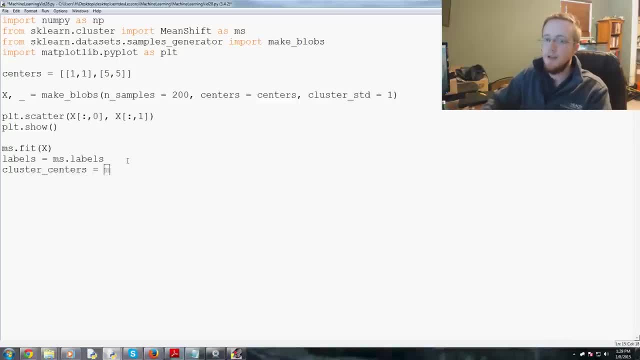 Now we're going to do cluster underscore centers And these are going to equal the mscluster underscore centers underscore. So these will be like the centroids, only not so much, But these will be the estimated centers. So again, it will be interesting to see how closely the computer predicts the cluster centers. 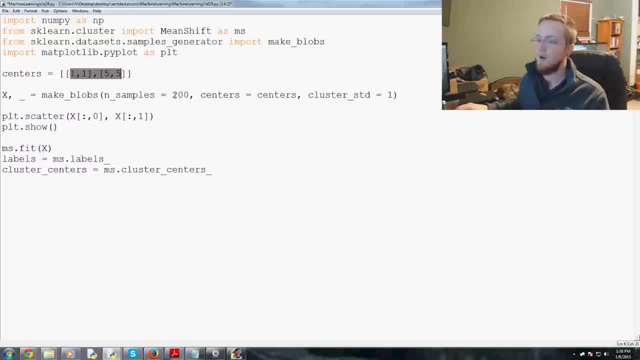 to what the actual cluster centers were. In theory, the higher we make the samples variable and the lower the standard deviation is, the more accurate this valuation will be in relation to the true starting number. Moving on Now, we're going to have n underscore clusters. 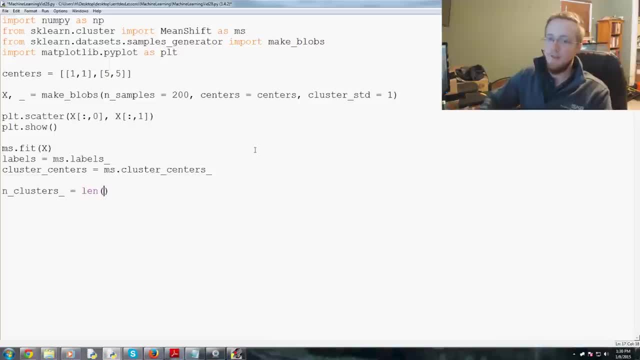 And the number of clusters is going to equal the length of the npunique. And what the npunique functionality does is it looks at an array and it tells you how many Unique variables there are, not what the unique variables are, but how many exist. 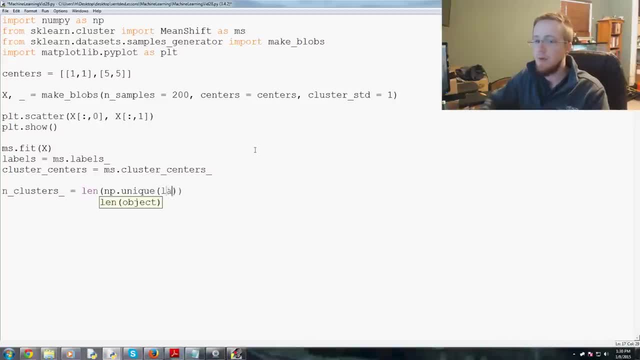 So npunique. And then we want that to be run on labels, And this will tell us how many categories or cluster types the machine has returned to us. Now what we want to go ahead and do is we're just going to print this out. 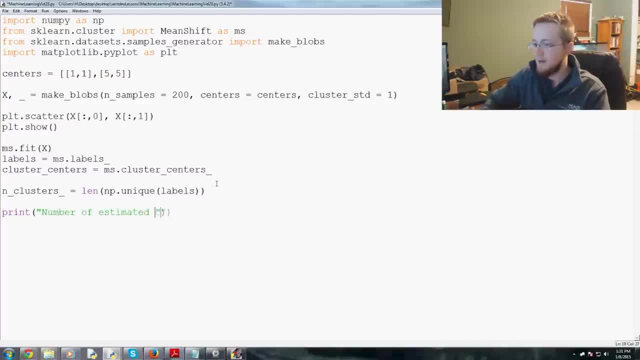 And we're going to say number of estimated clusters And we're just going to have that be n clusters Unplugged, So that just returns to us how many numbers or how many clusters, the number of how many clusters there are. 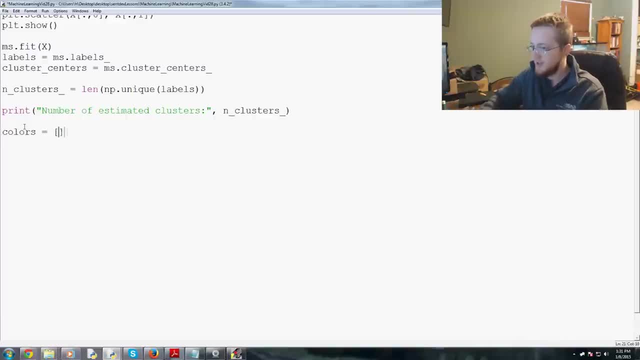 Now we're going to specify a list of colors for plotting. It'll be very similar to what we had used before, So we'll just kind of make a list that we're about to populate. now We're going to do r period for red. 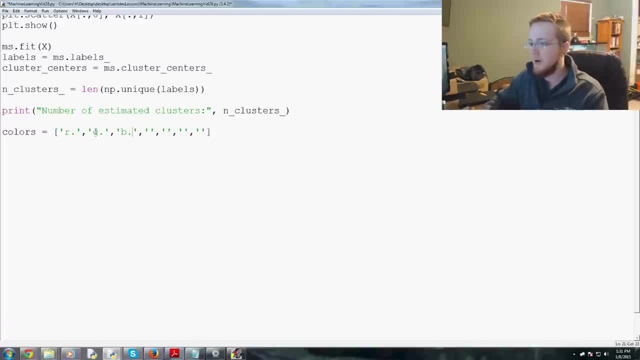 Green period for green Or g period for green, B period for blue, Then we've got c period for cyan, K period for black, W Or y period for yellow, And then we'll do m period for magenta. Now it's totally possible that we have more than these many clusters. 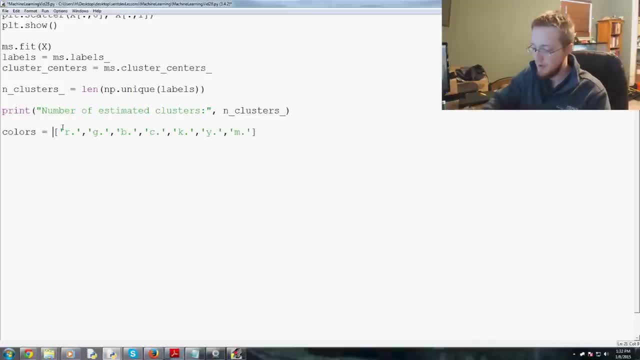 So just to make sure that doesn't become the problem, we're going to do 10 times, And what this is going to do is just make this list 10 times as big as it is. It'll just be repeating over itself. That way we won't run out of colors to choose from. 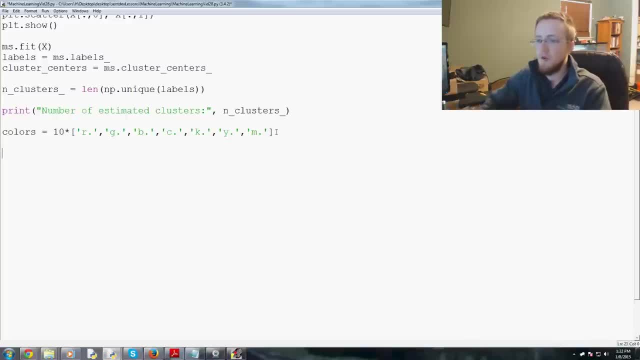 Hopefully, if we have more than 70 categories- something long. So, moving right along, We're going to go ahead and just so you can visualize what's happened there, in case you haven't followed, you can print out colors And then we'll also print out labels. so we understand it's a one-dimensional array. 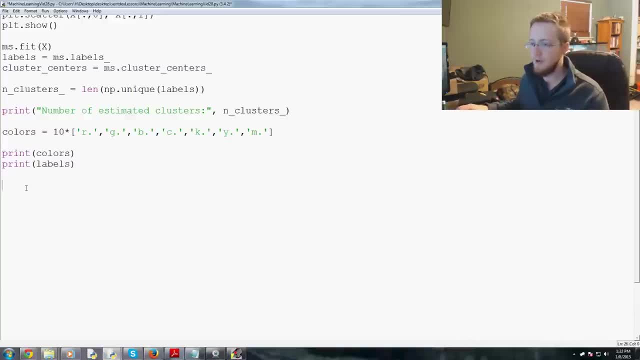 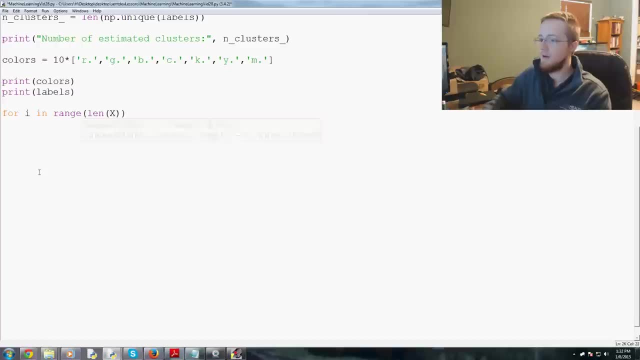 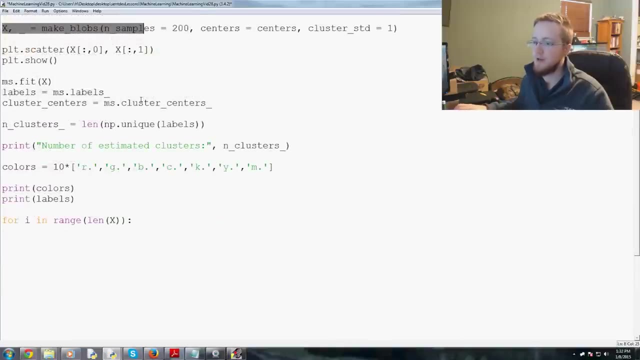 Now we're going to do pretty similar code to what you've seen before in the previous video, So none of this should be too new. So we're going to say for i in range of the length of capital X, So basically, for i in the range of this cluster data that we 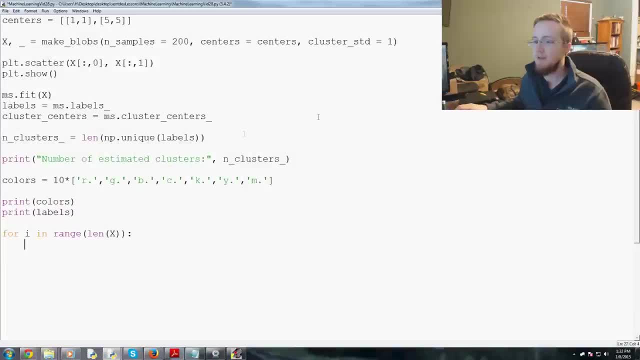 you know, generated. what do we want to do? And we have the labels that the machine has chosen in a list, So that will be a list of equal length to X, So we'll know what the corresponding label was. And now that label will be either a 0 or a 1.. 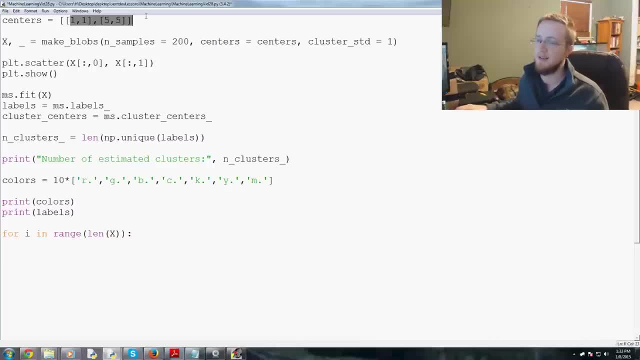 So then we can call or a 2 or a 3,, I suppose, if it incorrectly decides that there's more clusters than there are, And then we'll use that number and apply it to this list to pick what color to chart it in. 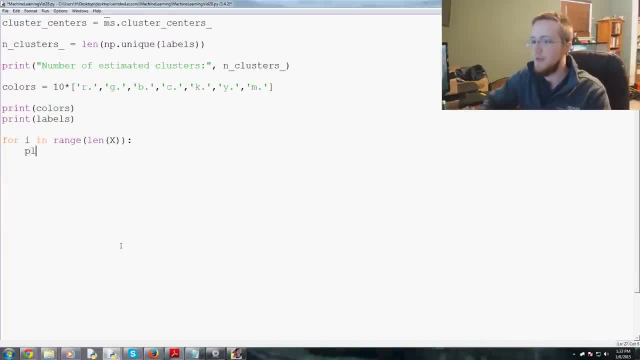 So for i, in len of X, we are going to dot plot, and again using similar syntax as before: the X, or the i-th of the X-th, The 0-th of the i-th of the X. There we go Anyway: X, i and 1.. 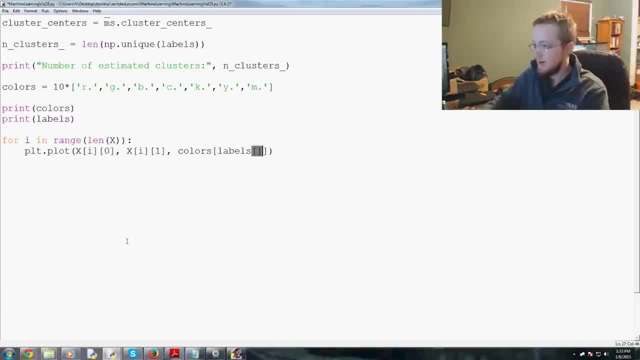 And then we'll say colors labels: i And that will be the you know one of these in this list. basically, Again, this is all similar syntax to before, so hopefully you're still following there. And then marker size: It will equal 10.. 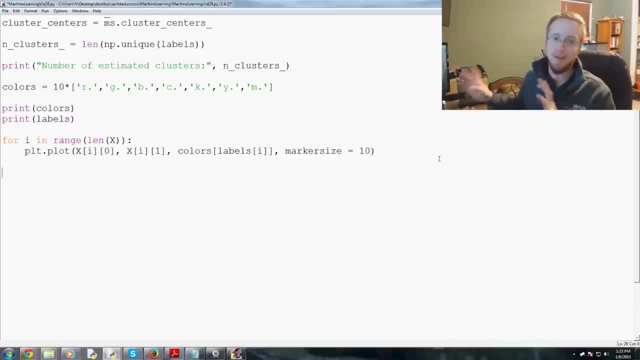 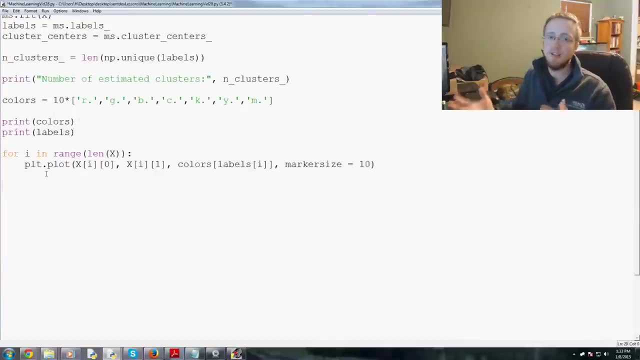 And that's it for this for loop. We don't really need to do anything else. We could print out the coordinate and the label like we did before, But we have 200 samples, so I don't really want to do that. Next, we're going to plot and scatter the center marker, right? 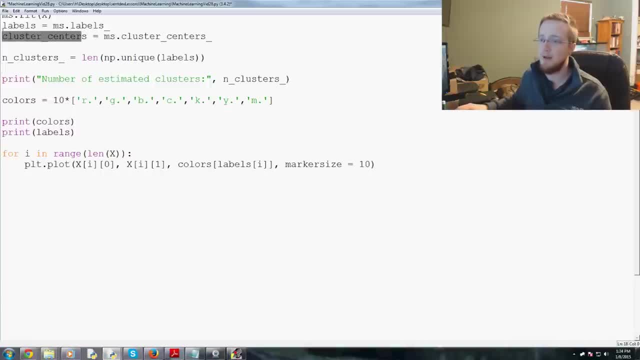 So we've got cluster centers, kind of like centroids- Not the same thing, but kind of like centroids, Cluster centers here- And so we're going to go plt dot scatter And we're going to scatter the cluster centers, And this will be using similar code that you've seen. 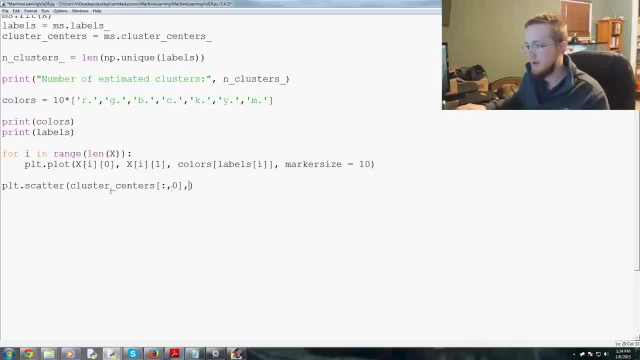 So colon comma, 0, comma. And then I'm just going to copy this so we don't have to type that all out again, And now we'll use the number 1.. Then we're going to say we'll hit enter here after that comma. 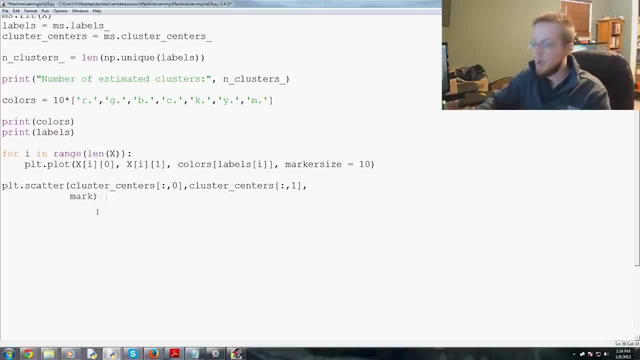 Don't forget your comma before you hit. enter there. Marker equals an X And the size will be 150.. The line widths will be 5.. And the Z away 5 and the Z order will equal 10.. Finally, we run plot dot show. 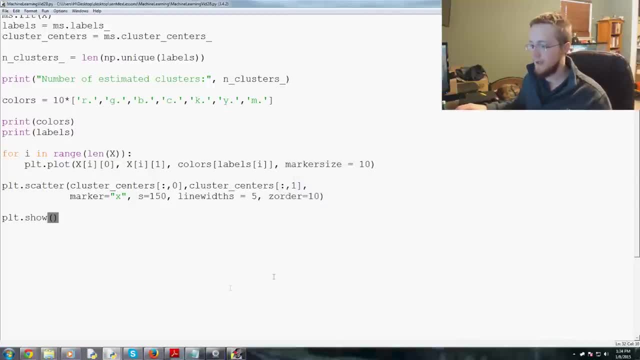 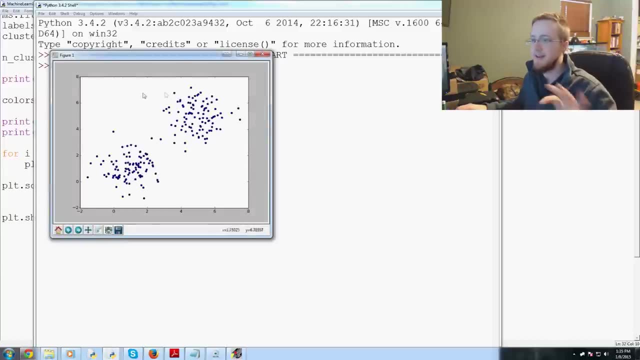 Save and run it And we wait a moment- hopefully not too long- for it to pop up. It took a while just to load there And here is the initial plot with the data, So we can see: okay, we've categorized this and this. 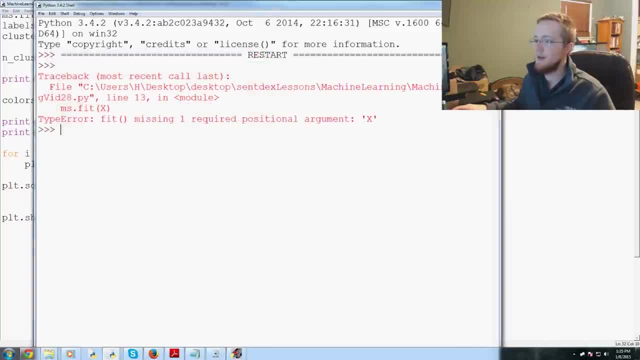 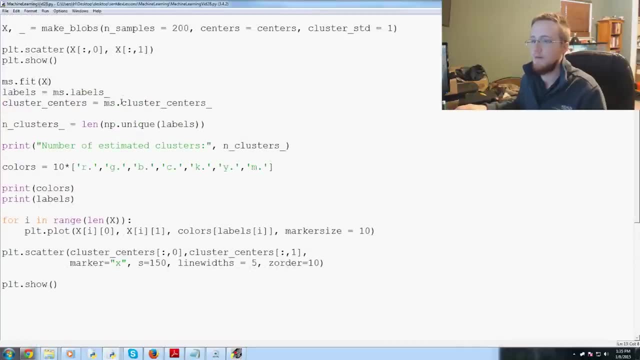 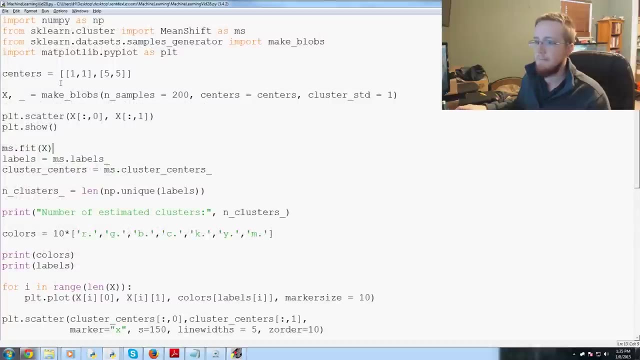 But we're not really sure about what to do with these center points. We'll close out of this. Did we not even put a positional argument in there? Well, we sure did. We put in the fit X there. Fit X, I'm looking at it. 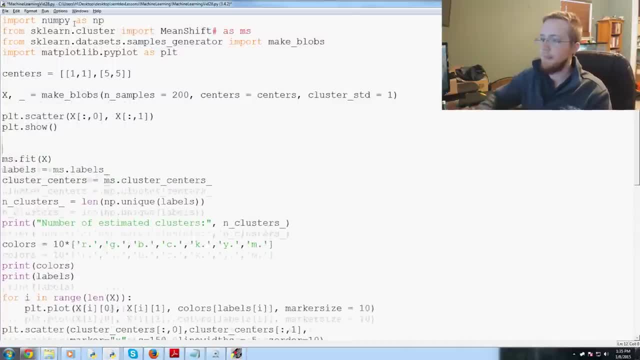 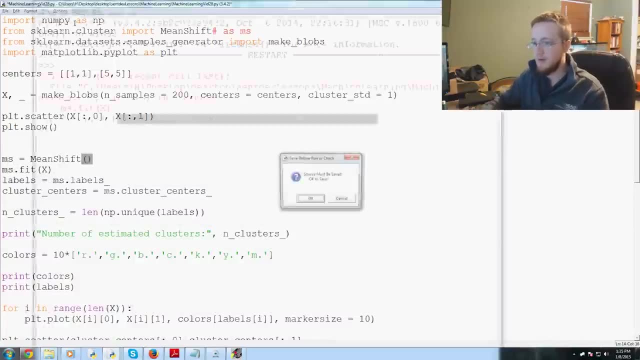 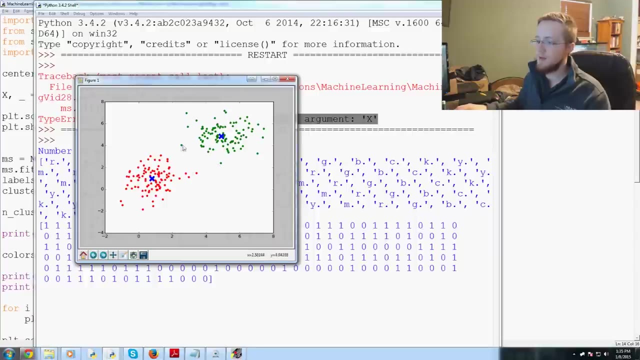 Let me try the following one. We'll say: MS equals mean shift, as follows: Let's try this one more time. There we are, Okay. So now we've got the plot. These were the center points. Now, this time I was mostly testing it. 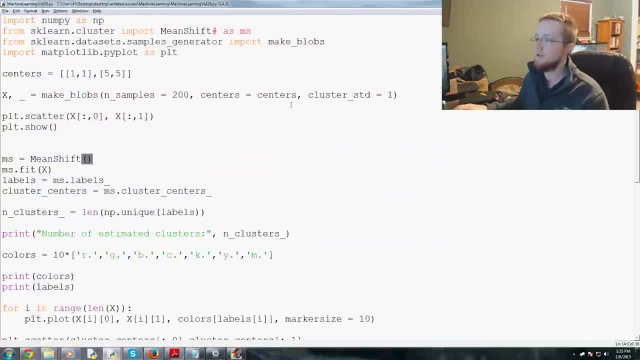 So we'll run this one more time and I'll explain what just happened, I suppose. So this was, I suppose, attempting to import it as MS And we were having a little bit of a problem there because we wanted to actually run the function itself. 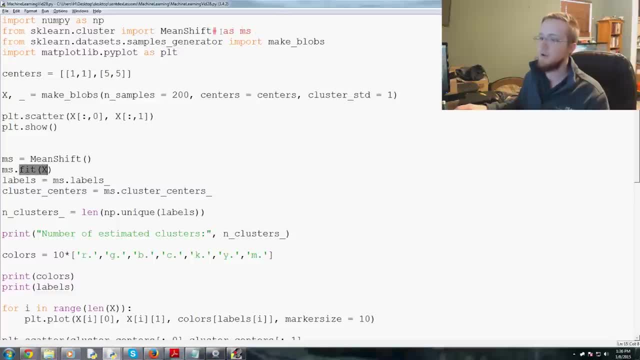 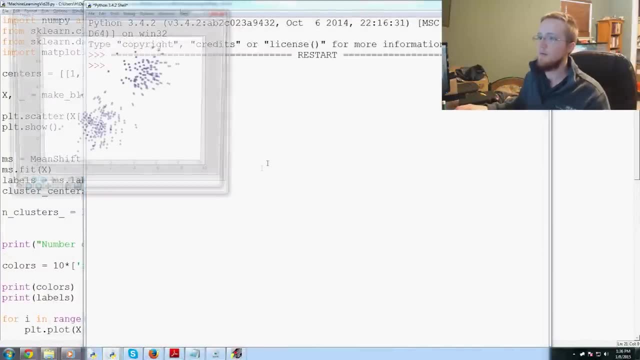 So that was kind of our problem. So it's this function dot fit, as opposed to just MS dot fit. So anyway, So now what we're going to go ahead and do is: we'll run that one more time, We'll run this one more time. 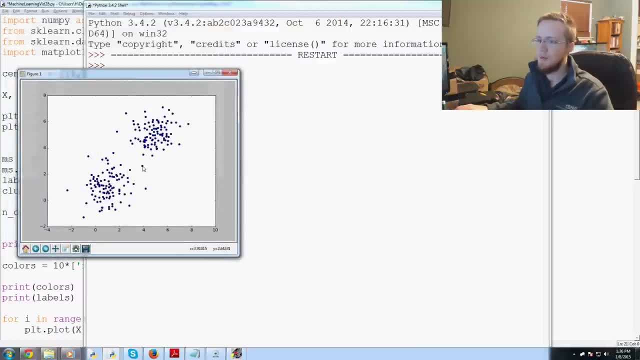 We'll see, we'll run this one more time. I think we're good, We're good, We're good. So now we're going to run this one more time. So this will run this one more time And it's going to have this pop up for us. 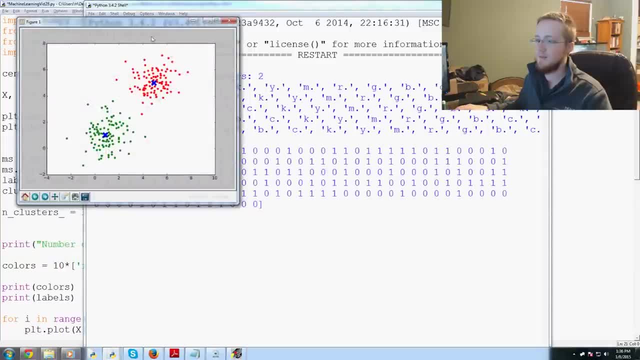 And so again, here's our two clusters And here's a center point that I would not know where to apply that. So, anyway, we'll close this and we'll see what the machine says. Okay, Well, the machine says it's part of this cluster here. 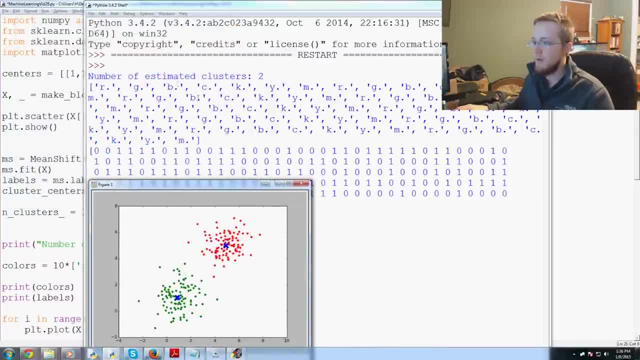 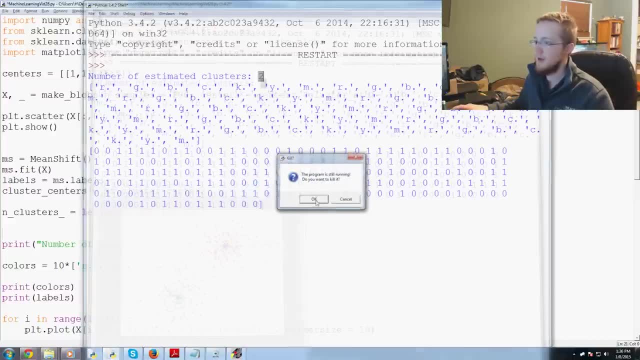 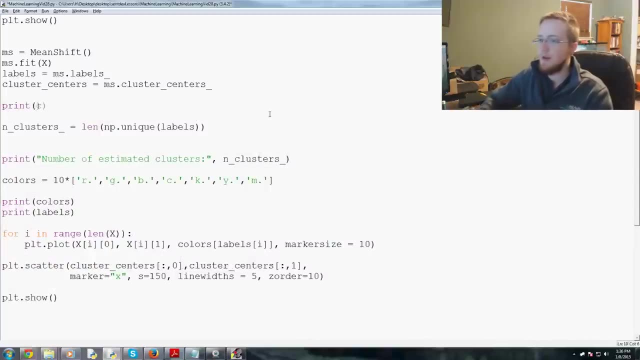 Interestingly enough, we can move this over here and we can see. okay, sure, the number of clusters is two. that it suggests. Ah, I meant to plot or print out the center points. Let's close out of this. Let me right here. we're going to print cluster underscore centers. 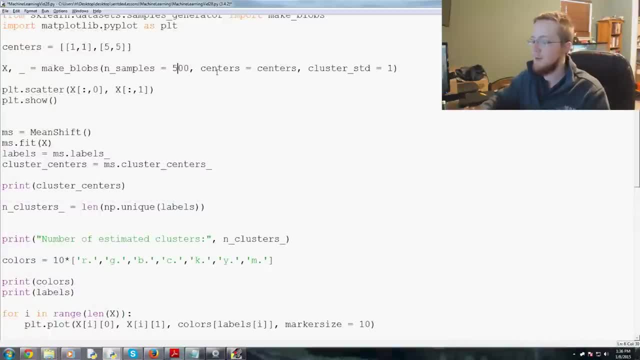 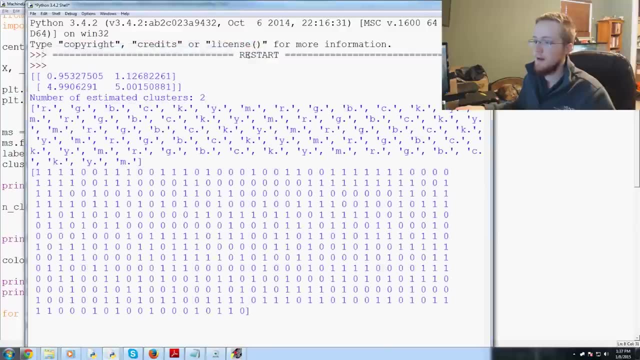 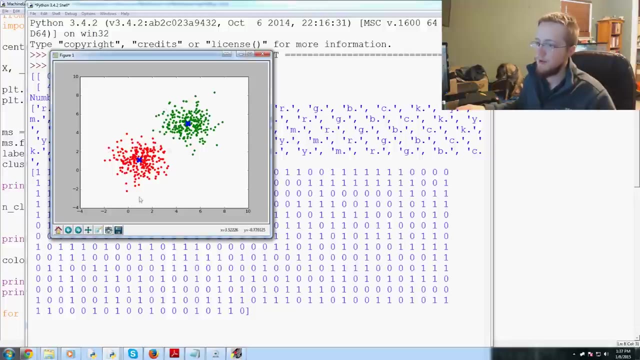 So now we can actually compare that to these centers. Let's raise up the number of samples as well. So this is the data. We'll close this And it runs, the test fits and all of that. And here we have a group here and another group here. 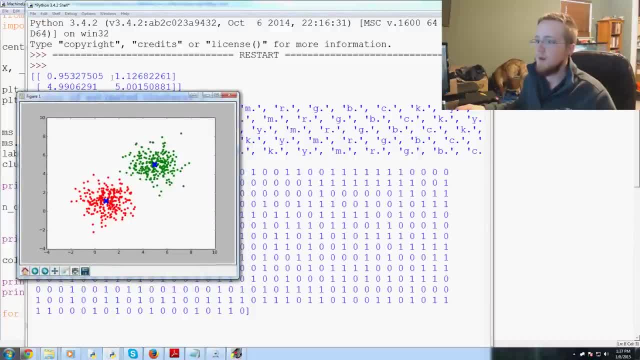 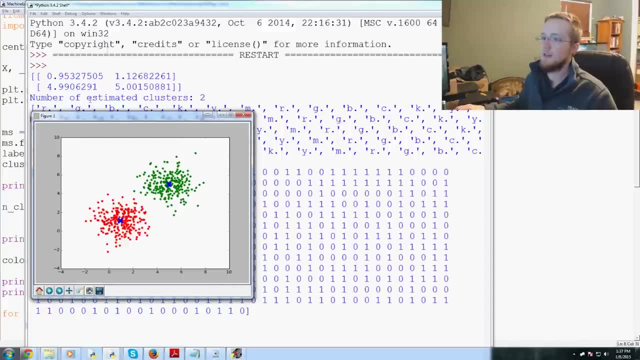 And now let's see what the centroids were. Well, we've got a 0.95 and a 1.12. And a 4.9 and a 5.00.. So yeah, that's pretty darn close to the initial 1.155.. 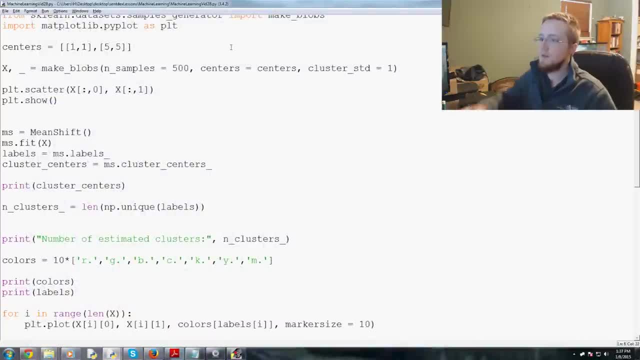 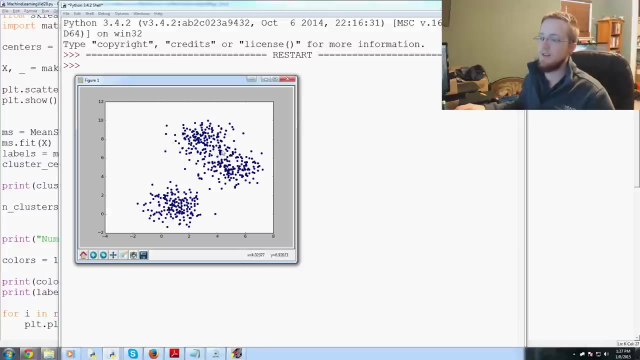 Now what happens if we, for example, say let's do 3.8.. Run that again. So here we've got what appears to maybe be a blob, But we can totally see how the center point could be right about there. 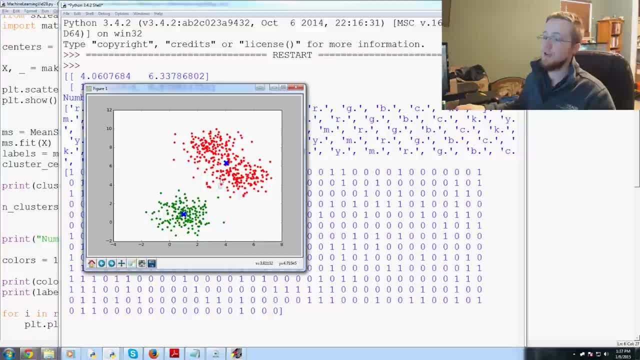 Let's see what the machine says. And indeed the machine agreed with me that that looks like it mostly is all one big blob And this is a second blob. Now there are some ways that we can tell the machine. hey, we want you to kind of be a little more specific in your categories. 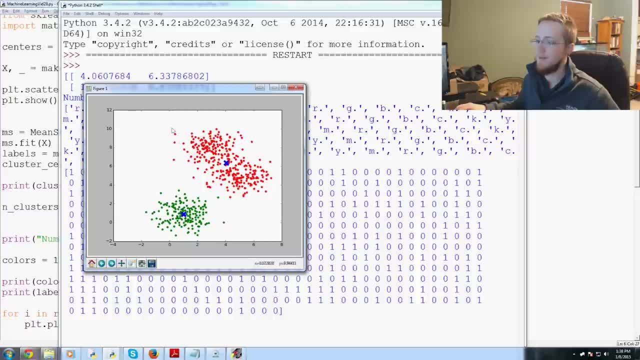 Or you want to be more like we would call this maybe a blob and this part of that blob, And this is pretty clearly a blob because there's even white space between them. But we can use it to create. We can use it to create a more, just like a more tight threshold, basically. 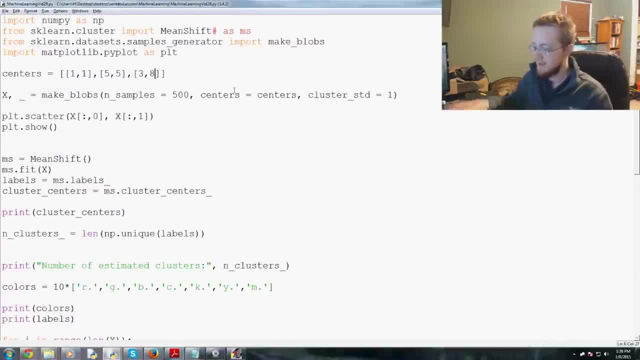 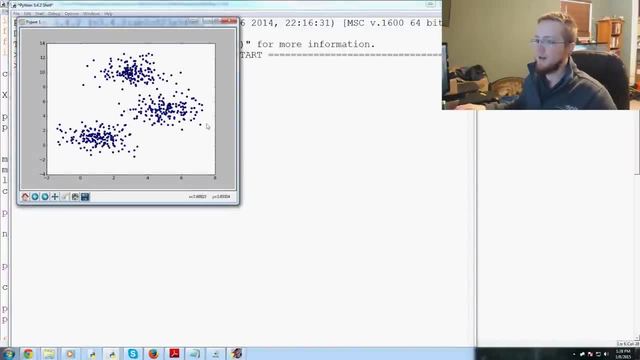 There's a lot of parameters that we can adjust here, And you can see why that becomes necessary. Let's do 3.10.. Let's see what this one does. So this is a little more defined. I can see clearly three center points there. 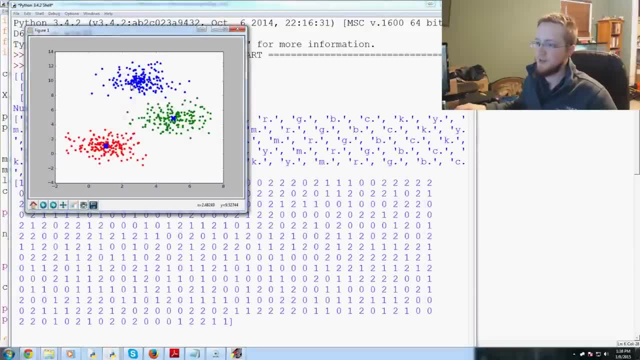 So hopefully it gives us three, And sure enough it does, Although the blue X. we cannot really see where the blue X is. That was kind of a silly idea. What were you guys thinking? Anyway, so now we've got these groups here. 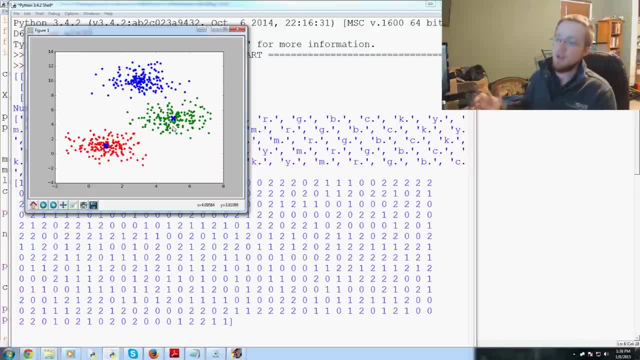 So So we can see that it indeed chose right. I mean, obviously this point could have been from this point and all that, But for the most part we can definitely see that this looks as we would expect And sure enough, 1, 1,, 5,, 5, and 3, 10.. 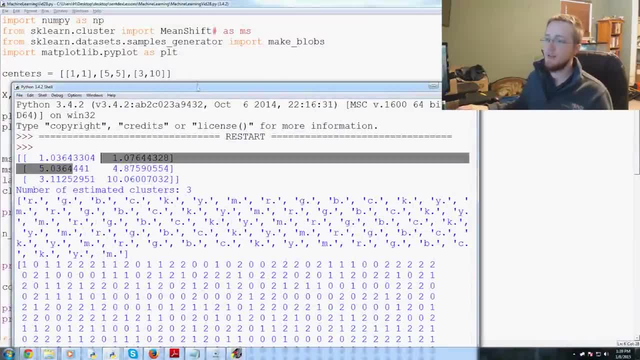 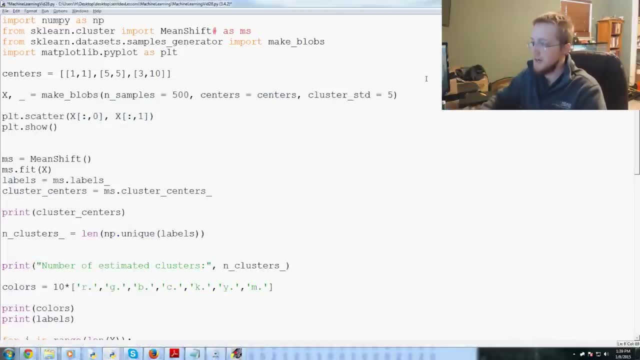 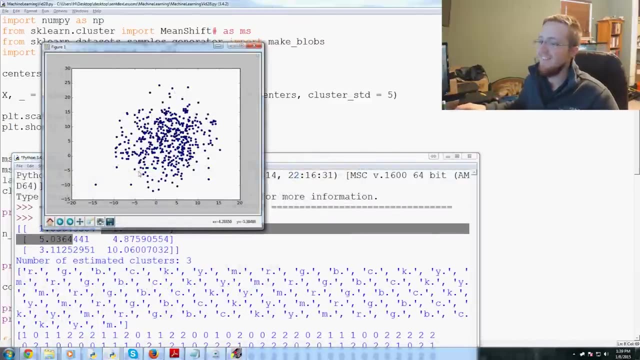 And that is exactly what we had pretty much chosen. So we can see that that seems to have worked pretty well. But of course we can always fool it by increasing standard deviation And getting the following: So how would you group this Right? 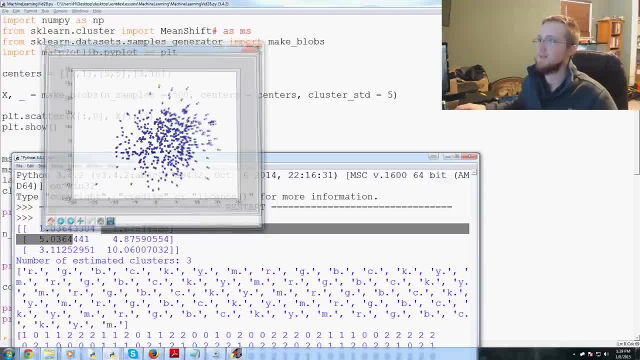 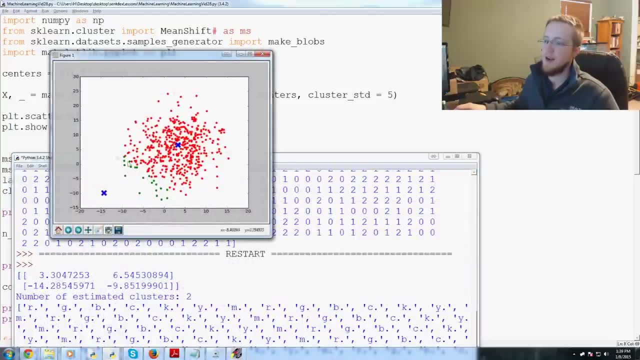 What are you going to do? Maybe you know, apply this as an outlier or something like that. We'll see what the machine says. Right? So the machine says, OK, this is clearly an outlier. These guys are closer to this little guy over here. 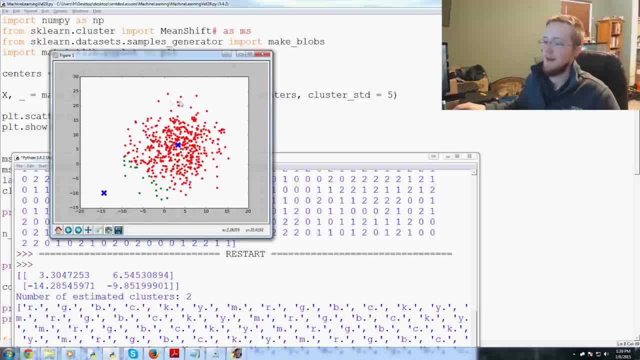 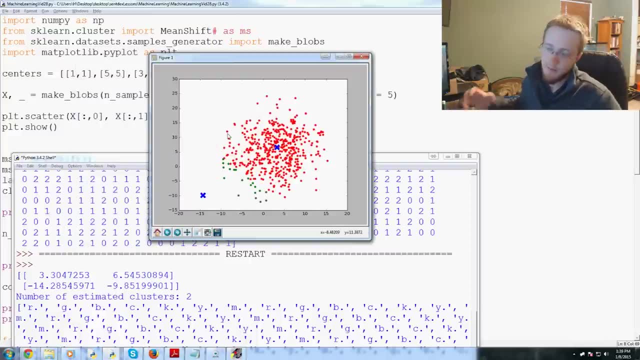 So it says, yep, that's a point of its own, And then everyone else is the same. So, obviously, when it comes to this, there's a lot of tweaking that's required Depending on what kind of data set you have. 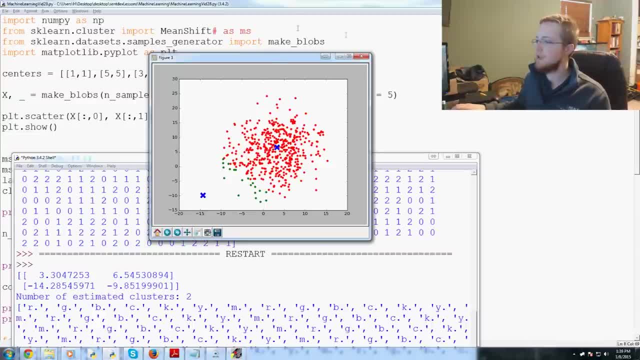 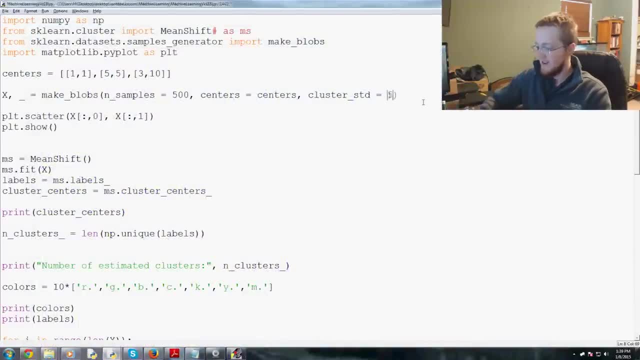 So- and that only makes the most sense- What we're doing is we're throwing data at the machine And we're basically letting it do everything. So it only makes sense that this is the more complex version of machine learning. And let's do a 0.3 just for kicks. 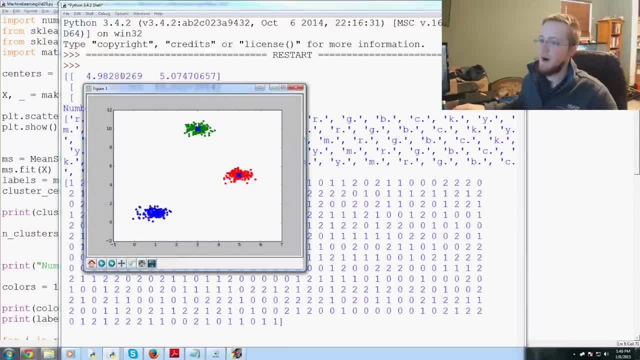 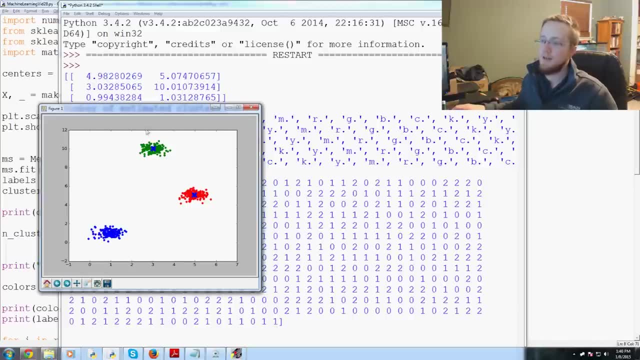 So obviously that's pretty clear And yeah, it's right on the ball pretty much. And again, you can see that accuracy as far as picking the center point is pretty darn high, Just simply, Just simply because of like what I was saying, the standard deviation went down. 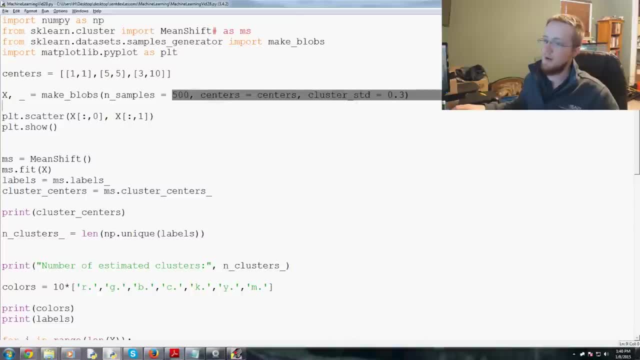 And if we rose number of samples to a higher number, it would only be even more accurate. Anyway, that's it for the basics of this. Like I said, as you can see, this is only going to get more and more complicated. 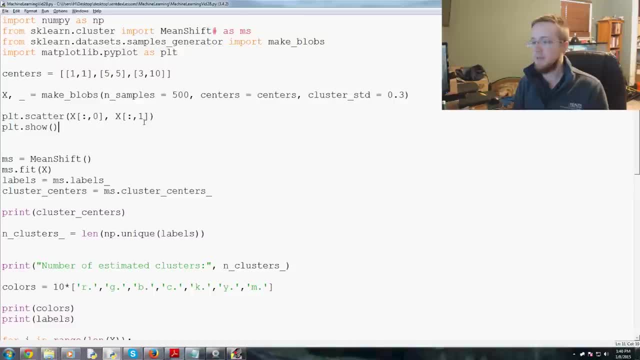 Especially when it comes to unsupervised machine learning And allowing the machine pretty much full ability to determine what is actually different In the data. So we can see that it can be quite accurate And it's very good if you feed it the correct amount of data. 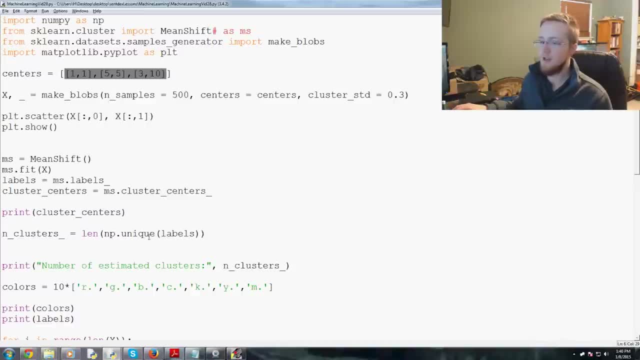 And later on we'll talk maybe a little bit more about some of the parameters that you can specify, Especially in mean shift. here as well, There's a lot of default parameters that we haven't covered. So anyways, basic covering of it.